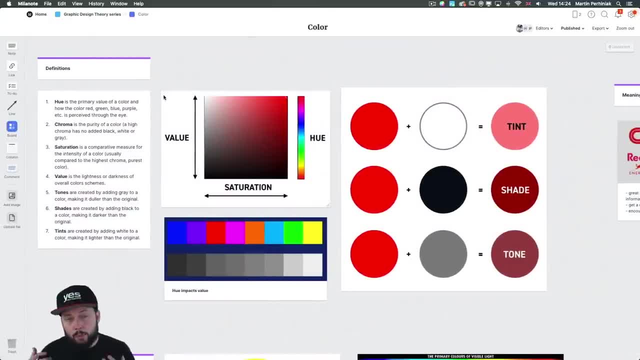 about definitions first. So you probably heard of hue, saturation and value or brightness. Now, these are quite basic things that you most likely know already if you are using any of the Adobe applications. Most applications would show it as a vertical bar, but it can also be. 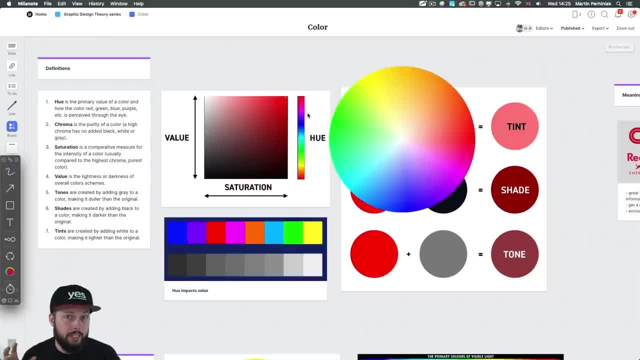 represented with a 360 degrees color view, And that is why normally, when we refer to hue, it would be 360 numbers, which represents the 360 degrees of a full circle. Saturation is a term that you probably again heard of, and this is an important one. 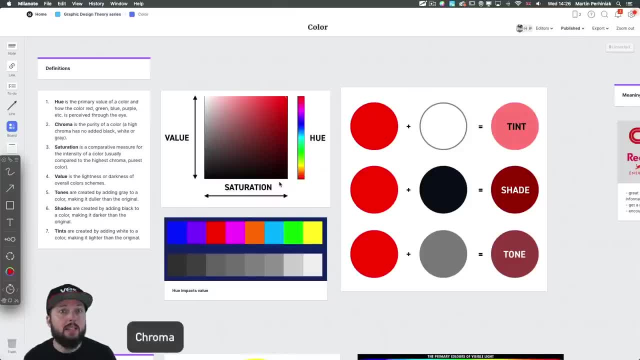 but probably not as important as Chroma. Now, Chroma is the term that we normally use to define the purity of a color, So the highest chroma value you can get when you have a color without mixing with anything else. So, for example, red, a complete red, would be the highest chroma. 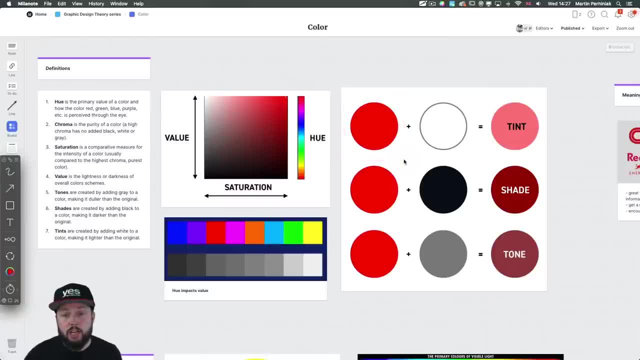 you can get And then, once you start introducing different shades to it, like white, you will end up having this chroma. So chroma would be the highest chroma you can get. And then, once you start different tints of red, or if you mix black, you would end up having different shades of red and 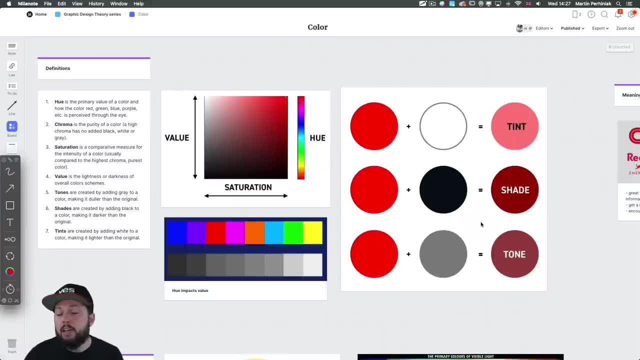 finally, if you add gray- any type of gray- you will end up having different tones of red. and when we talk about saturation, it's slightly different because it's more of a comparative measure where you would compare the intensity of a color to the most vibrant or highest intensity color which we 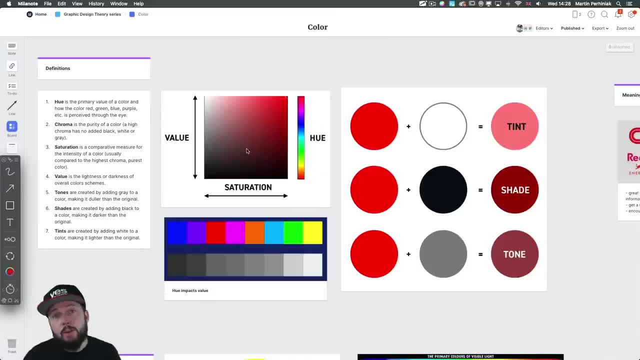 would normally set as 100. so if you imagine the color picker in photoshop as a coordinate system, saturation would be the x-axis and the y-axis would be brightness or value, which defines how bright or dark a color is. now, so far it sounds fairly simple, but it gets complicated because 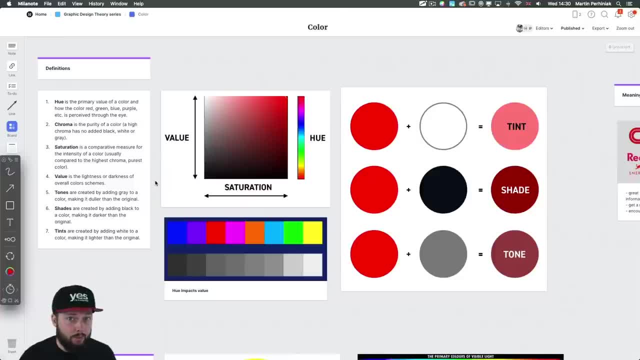 hue can actually affect and impact the value of a color and there is a perfect example here. so you can see the color picker in photoshop as a coordinate system and if you imagine the color on top and then below it, you can see their values. so even if you pick only pure colors, 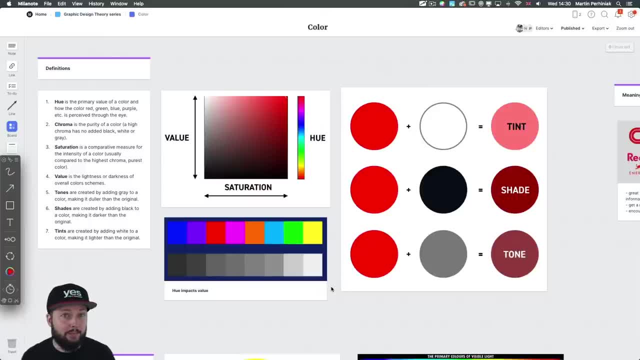 with their highest chroma, you will still have differences in their value. yellow, for example, is a very bright, high value color. compared to this, darker blue is very low in terms of value. so try not to confuse value with tint, shade and tone, because even without mixing white, black or 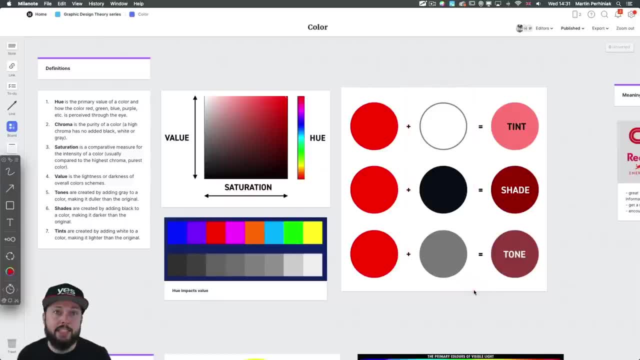 gray into the pure colors, you would still have differences between the values, and that is why it is so important, when you are choosing a color theme, which colors you pick, because you can end up having a low-key or dark composition if you pick darker colors or a vivid and bright composition. 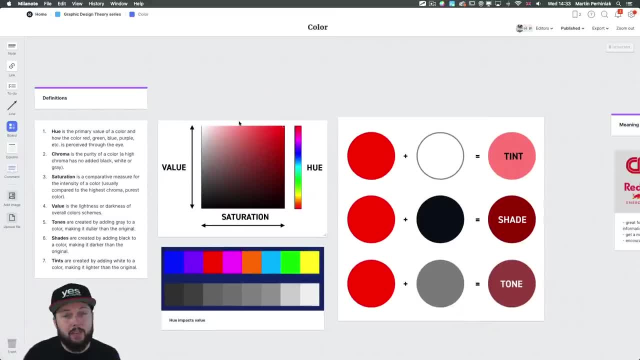 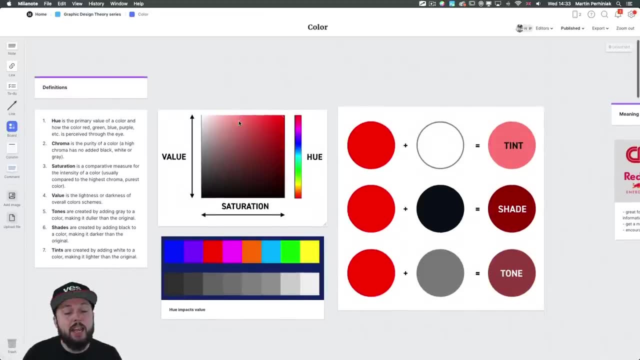 if you pick brighter or higher value colors. soon i'm going to show you plenty of illustrations and examples which will help you to make more sense of these terms. but first i would like to borrow a little bit of your time to show you how to make a color palette with just a little bit more science. 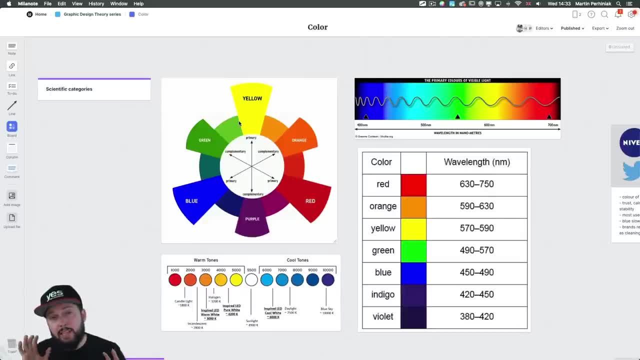 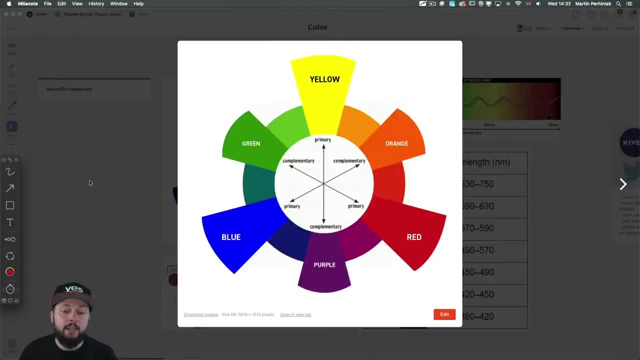 because i feel like this is also very important when we talk about colors. now, the probably the easiest diagram here that you can understand is that color wheel that we mentioned earlier. in this particular one, you can see the primary colors highlighted, so these are the ones that pop out. 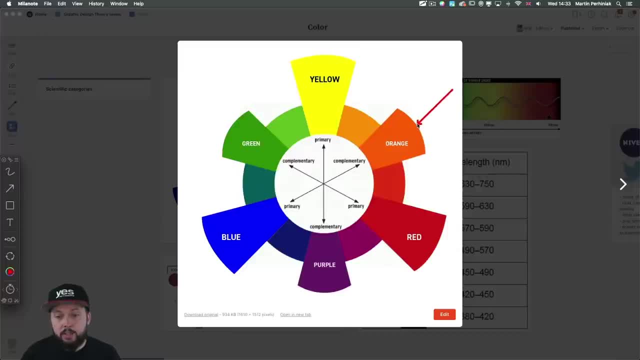 the most from this circle. then we have the secondary colors, which are always a mixture of the primary colors. so orange, for example, is made up of yellow and red, or green is made up of yellow and blue, and finally, purple is made up of blue and red. once you start mixing secondary colors with 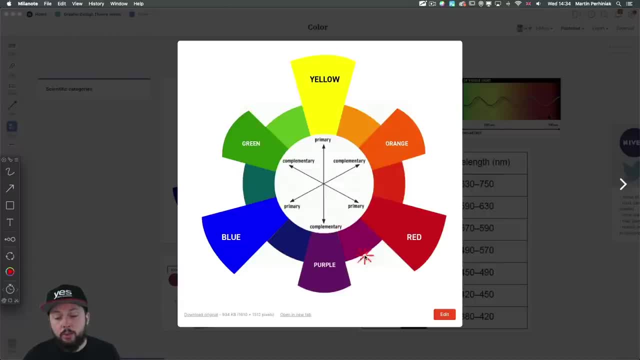 primary colors, you would get tertiary colors, and those are the ones on this circle closest to the center point. now, as a designer or illustrator, the color wheel is also important for you to be able to find color harmonies. but, most importantly, you can also find color harmonies that are: 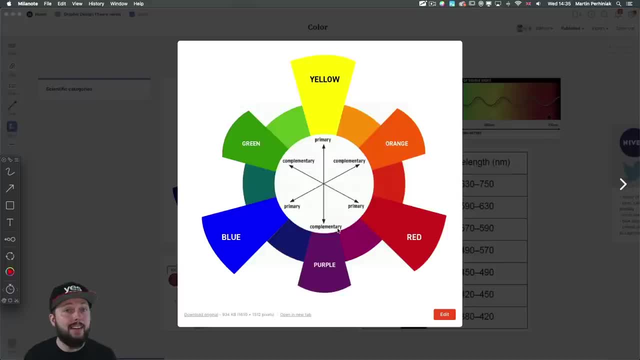 complementary with the primary colors. these are great color pairs and they work really well together. so the way you can find them is very simple. where you have, let's say, yellow, you just go to the opposite side of the color wheel and you will find the complementary color, which is purple. 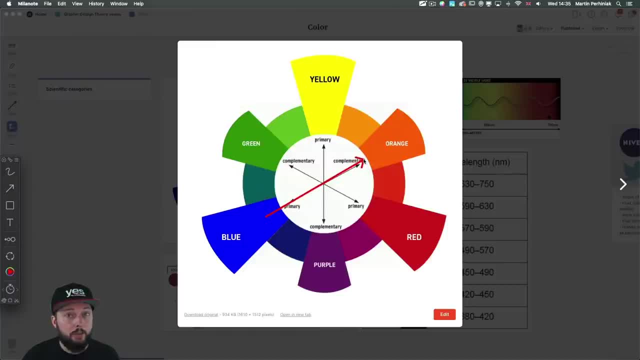 or the same thing: for blue the complementary color will be orange and for red is going to be green. so this is already a color harmony, but we will learn much more about this and all the other different types of harmonies between the complementary color wheel. first, let's see how red and blue work really well. 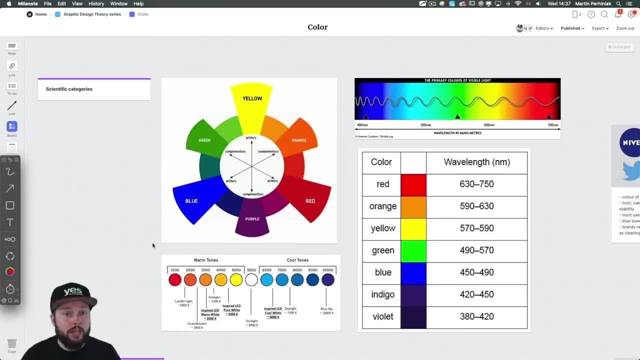 colors. Now, besides the color wheel, we can also categorize colors based on temperature, and that's what you can see here at the bottom. So it's measured in Kelvin, and the lowest values are the warmer tones, while higher Kelvin values would be the cooler tones. In the middle we have white, which is 5500 Kelvin, and 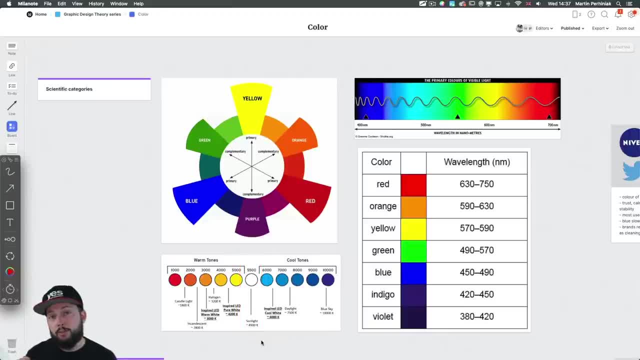 sunlight is actually a little bit lower than that: it's 4900 Kelvin. Now, this way of categorizing colors is more important for film and photography, but still, as a designer or illustrator, it's good to know that this is just another way of categorizing them, And I could get much more scientific than this if we 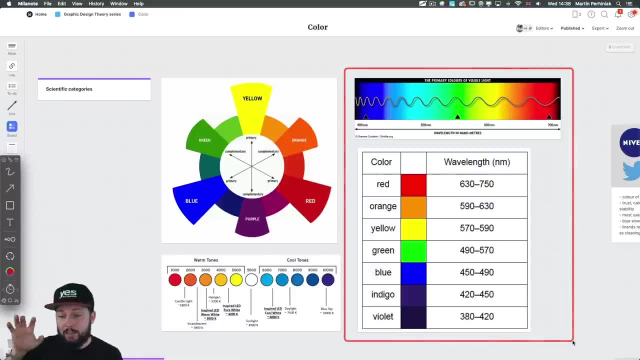 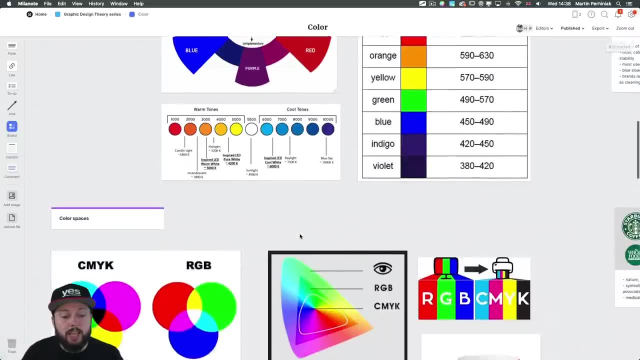 started talking about wavelength, but once again, when you compare the color temperature and the wavelength, you probably can already see the similarities. But let's move on and talk a little bit about color spaces. As a designer, this is definitely very important for you. as a designer, this is definitely very important for you. 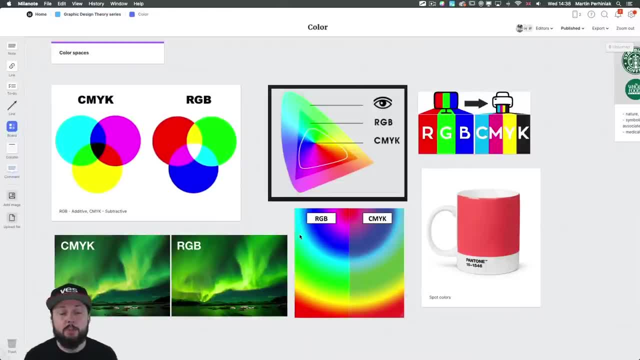 and most likely, you are already familiar with the differences between CMYK and RGB. So these are two color spaces used for different medium. while RGB is mainly used with devices that needs light to represent colors like a projector, camera and monitor, CMYK would be used for print and this diagram here shows it really. 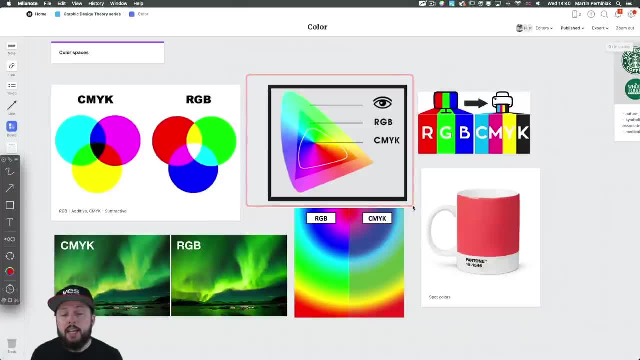 well that the visible spectrum of colors is actually larger than RGB and CMYK, and RGB is also larger than what we can represent with CMYK or cyan, magenta, yellow and black ink. It might be also useful to remember that CMYK is called a. 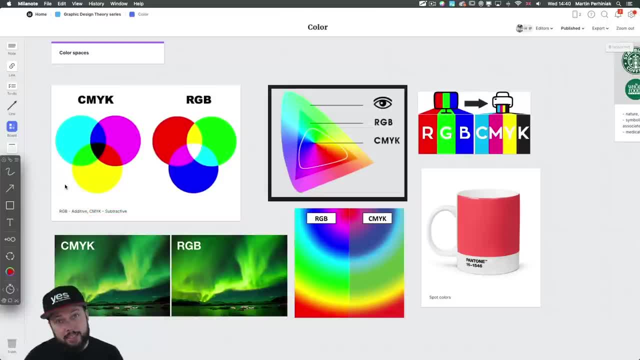 subtractive color method, where you are starting with white, so that's just simply the color of the paper, and then you are subtracting from it until you are getting to black, which is the most intense color when it comes to print. On the contrary, RGB is an additive. 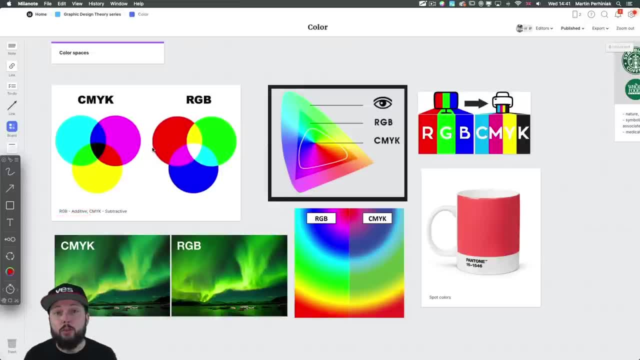 color method, where you end up having white when you combine or mix all the colors together. Generally, what you need to remember is that the colors that you see on your screen are not going to be as vivid and vibrant once they are printed, So this is what would normally happen once you 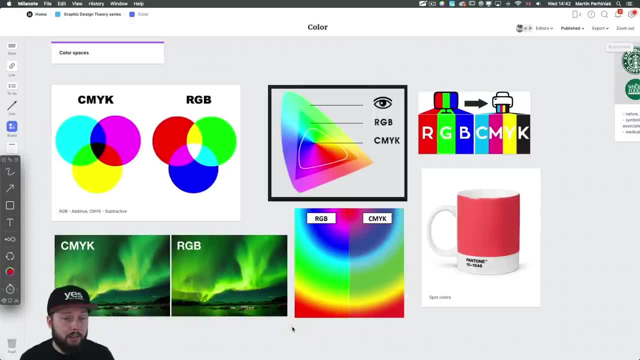 print an image out, it gets a bit desaturated and the colors get slightly washed out. This is again because of the difference in the spectrum. once again, all of these vibrant colors, in these corners, like here and also here and there, they are the ones that CMYK cannot represent. And again this: 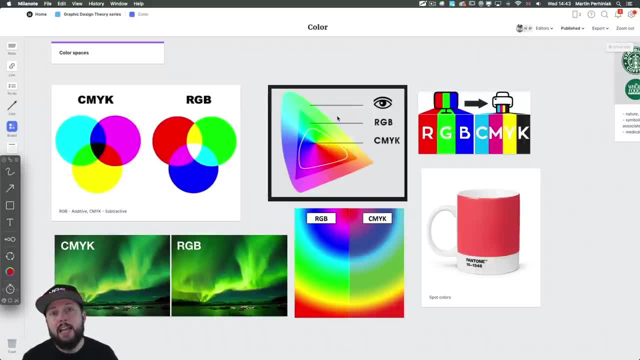 is a huge topic. we could talk about ICC, color profiles, color management and spot colors, but I am not going to go into too much detail. once again, I will cover these in the course that I mentioned earlier in the beginning. But, moving on, I want to show you something extremely important. 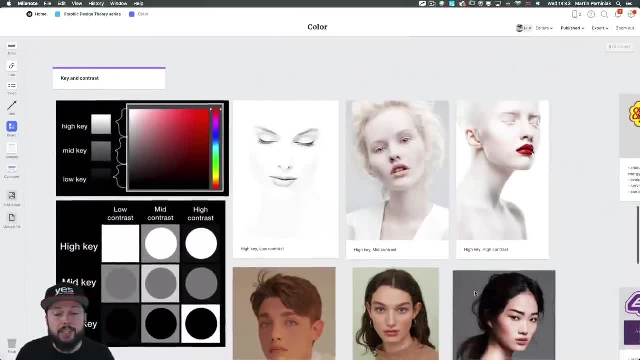 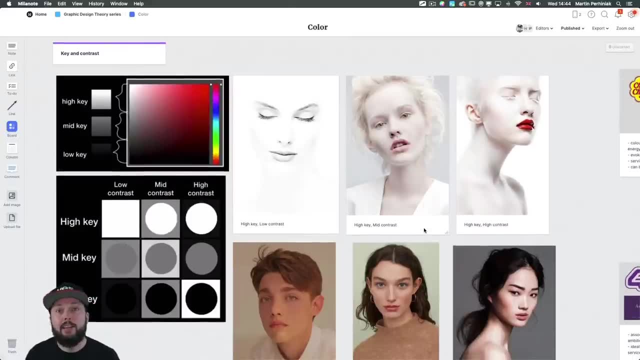 This is something that took me years to figure out and understand. the importance of. This is key and contrast, and these are two terms that normally you would hear separately, but once you start thinking of the two together as a pair, that's when it starts to make sense, and that's 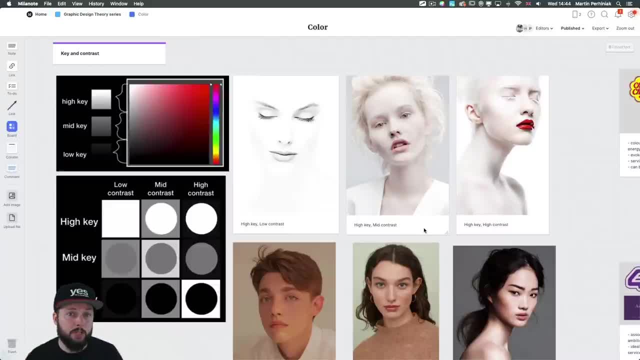 when it will help you creating really striking compositions, whether it's photography, illustration or graphic design. So both of these terms- key and contrast- has something to do with the value and you can see here on the top that the top third of that coordinate system would represent the high key values of colors. then we have mid key or mid tones in the center. 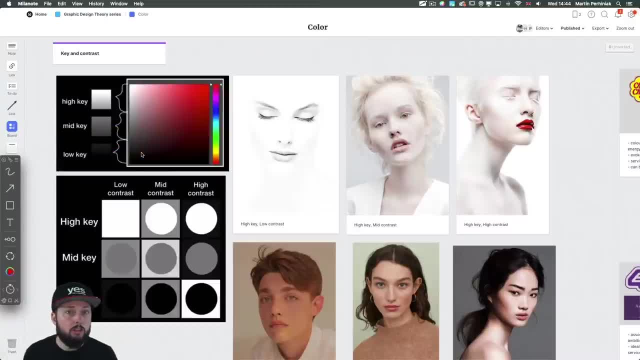 and then low key or darker values at the bottom. And contrast, again you probably are already familiar with, means that you have colors next to each other that are clearly different from each other. The higher the contrast usually the more striking that difference is, And here is a very interesting chart. 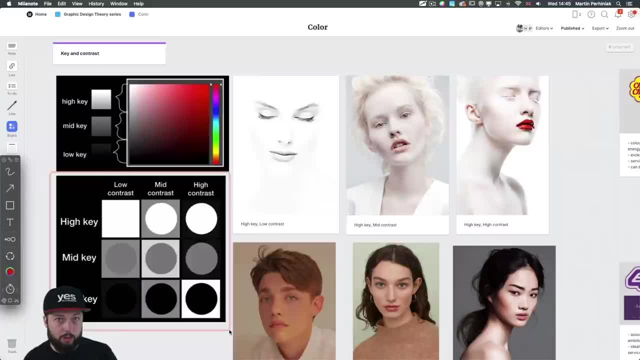 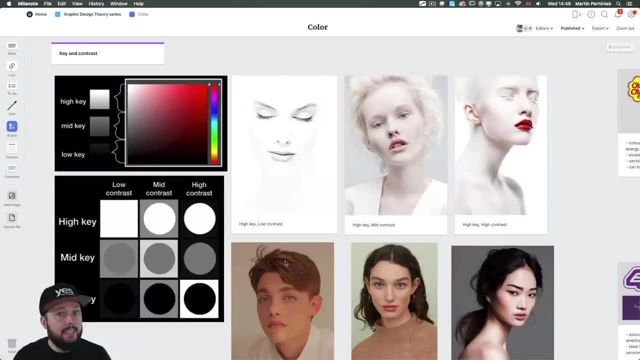 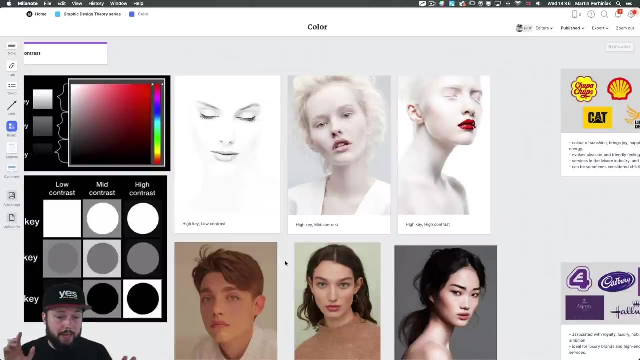 which shows the combination of key and contrast just simply by using grayscale values, but of course this would also apply to color images. And to make this easier to understand and to visualize it better, here are a couple of portraits showing exactly the same pairing of these two terms. So on. 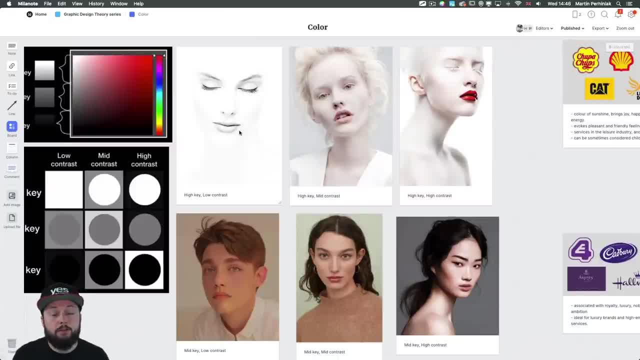 the top left we have the high key low contrast, followed by high key mid contrast and finally high key high contrast image. So they are all very bright, so the value is high, but we are increasing the contrast and mainly in this case the lips are the standout feature on the right side, It almost 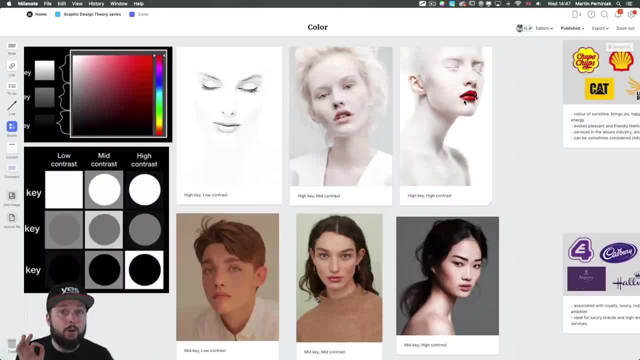 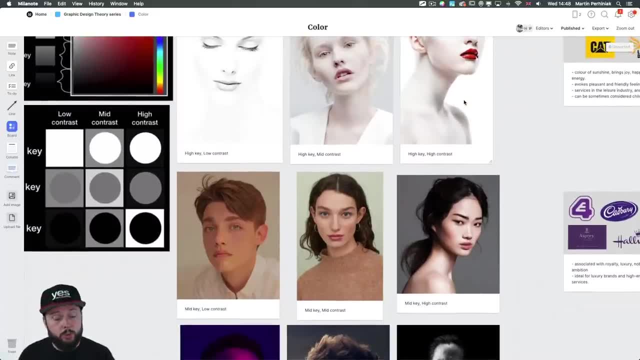 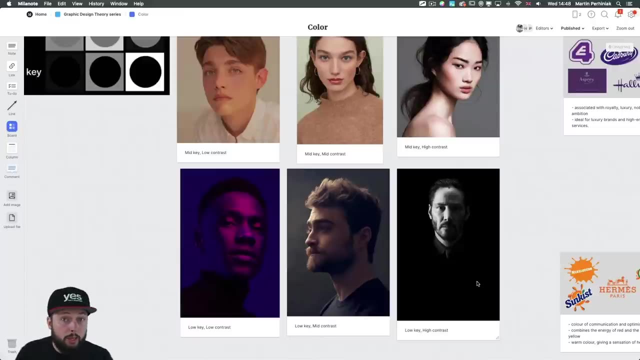 feels like it wants to jump off the screen, and that is how contrast can be used as a focal point in a composition. Further down we have the medium key row, again from left to right, increasing the contrast, And finally, in the last row, we have all the low key portraits, and similarly, here we have 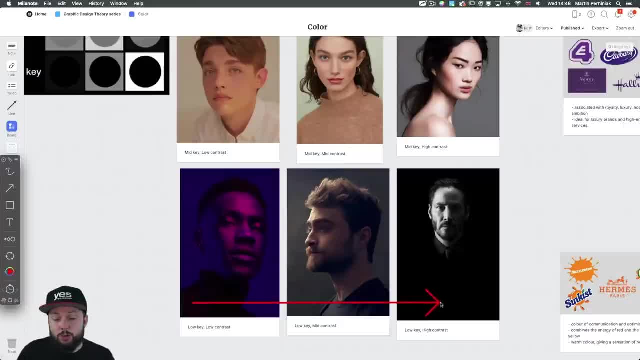 low key, low contrast on the left, and then we reach good old John Wick on the right with low key, high contrast. Now, these type of images are usually the most striking ones, because you have a lot of black and then you have some powerful bursts of white in certain places And, of course, the highest contrast you can achieve in a composition. 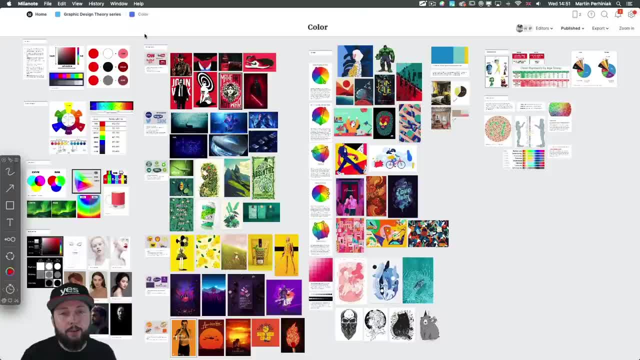 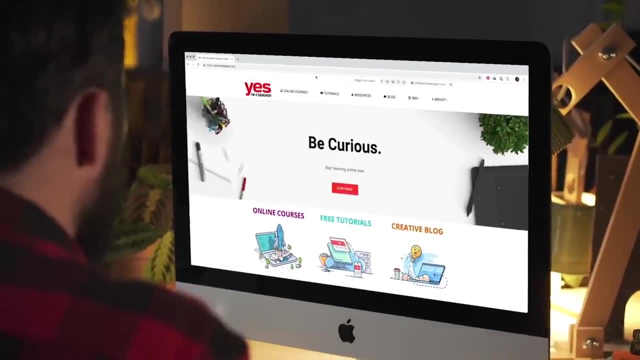 is pure black next to pure white. Alright, so now that we covered the basics, or fundamentals of colors, let's talk about the meaning of color, and this is more color psychology, and this is where we start to see some interesting examples. Before we continue, I just wanted to let you know about our creative 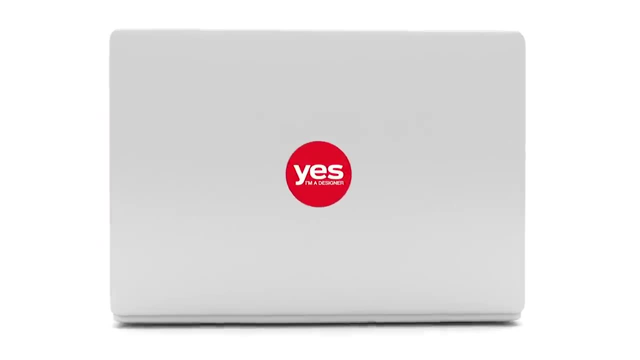 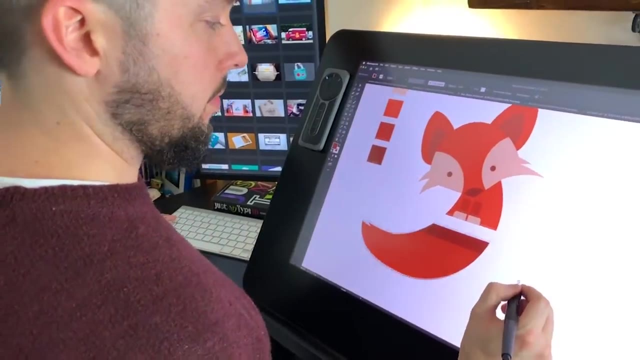 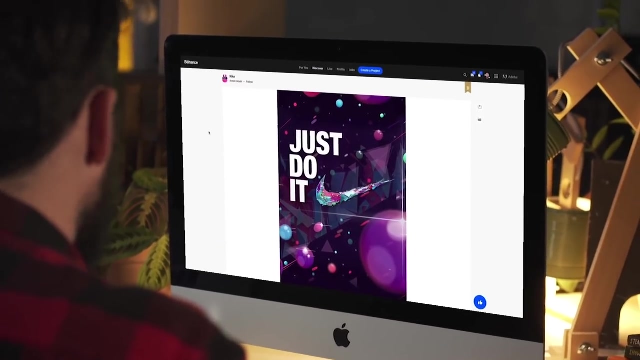 membership program. For a small monthly fee, you get access to over 200 hours of Adobe certified online training courses. Master all the tools and skills needed to become a professional graphic designer or illustrator. As a pro member, you will get mentoring from me and my team, access to 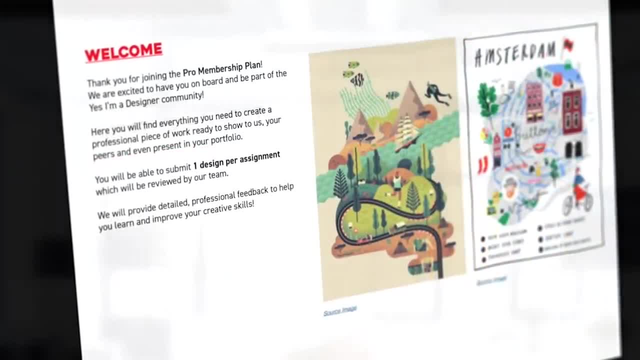 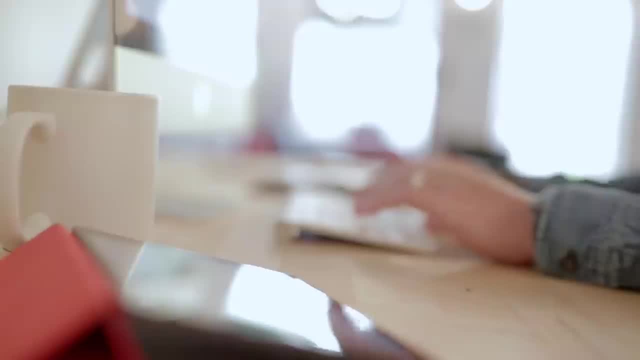 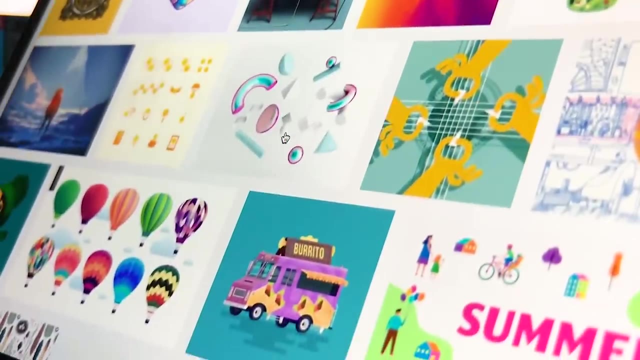 webinars, student forum and creative briefs To help you build an outstanding portfolio. Pro members can also download the project files for all of our YouTube tutorials. Sign up at yesimadesignercom, slash memberships and start your free trial today. And now let's head back to the tutorial. 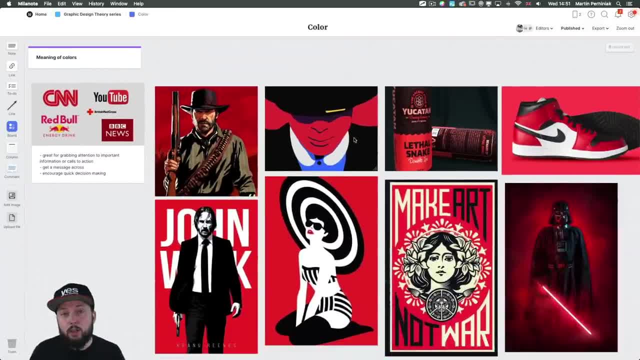 First, here is red. Now, if you want to learn more about the meaning of red, I actually have a separate video on that, which you can again find in the description below. And, in a nutshell, red is great for attention. It's a very striking color, especially when it's combined with black, and 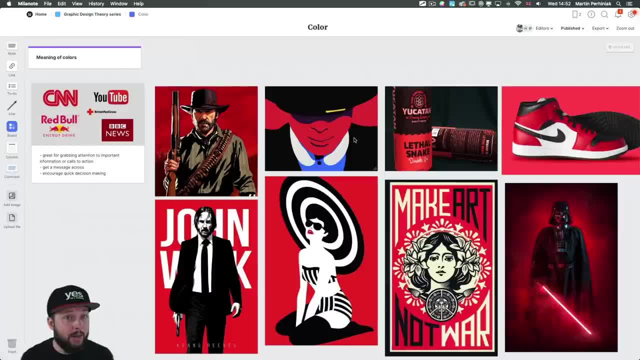 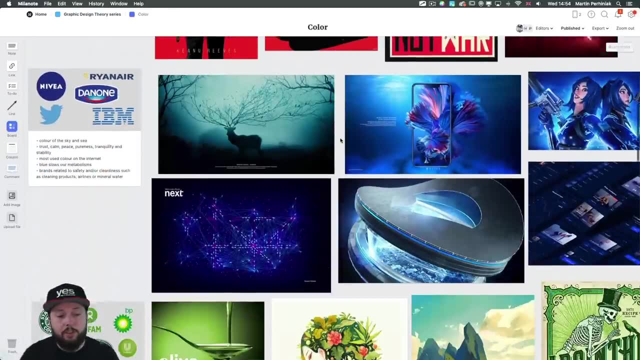 white And it can carry a lot of meanings, from power, aggression and strength to lust, fertility and- in some places the world, also prosperity In general, when you use red in your composition, it can help to make decisions quickly. It's almost like a call to action Moving on. we have blue. 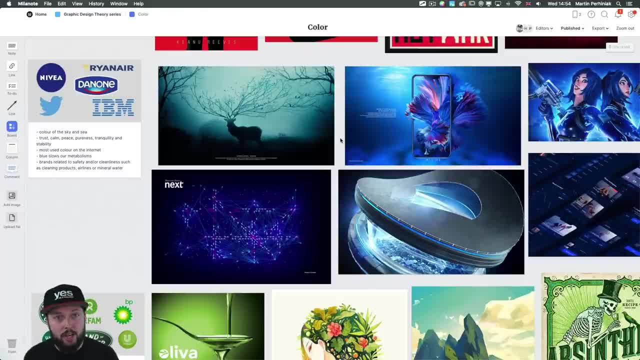 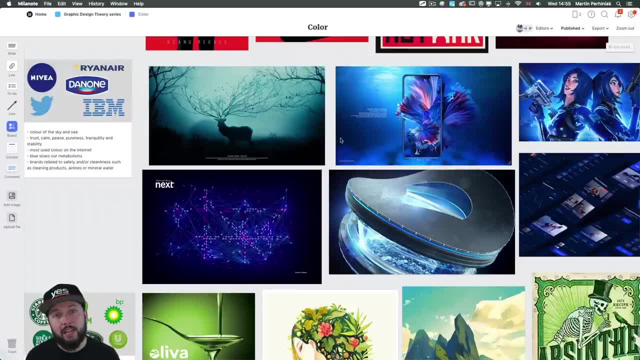 which is the color of the sky and sea, So naturally it would have a calming effect, but it can also represent trust, pureness, tranquility and stability. It is actually the most used color on the internet and amongst corporations, Especially for brands that are related or 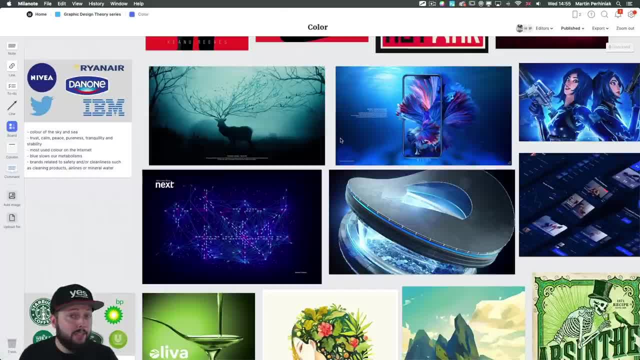 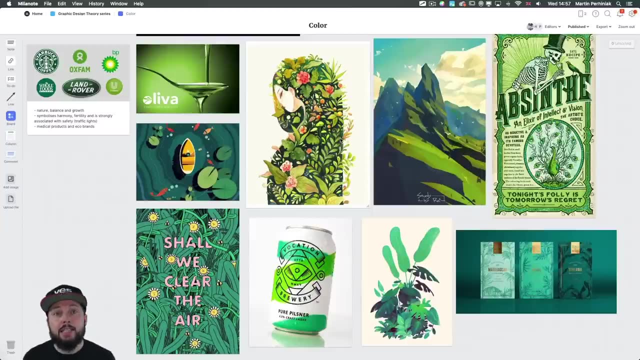 associated with safety and cleanliness. An interesting fact about blue is that it actually slows our metabolism down, So that is again why we consider it a calming color. And moving on, we have green, which is associated with nature, growth and balance. It symbolizes harmony. 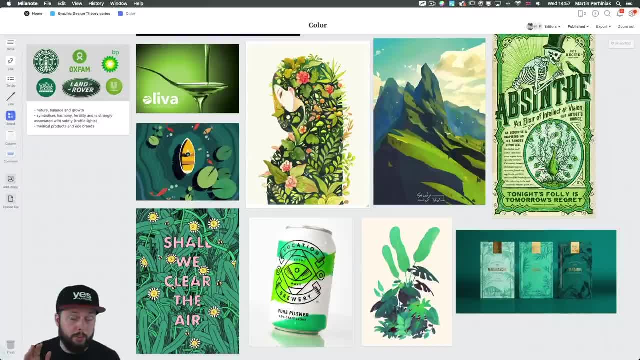 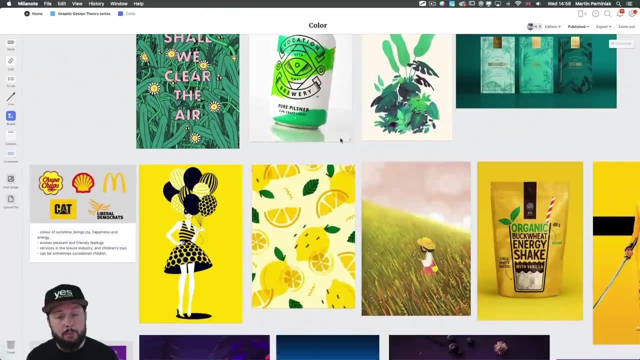 serenity, and it can also be used for safety, just like blue. Just think about the green man in the traffic lights. It is a color definitely often used by medical and eco brands. Moving on, we have yellow, which is the color of sunshine, and it usually represents joy, happiness and energy. 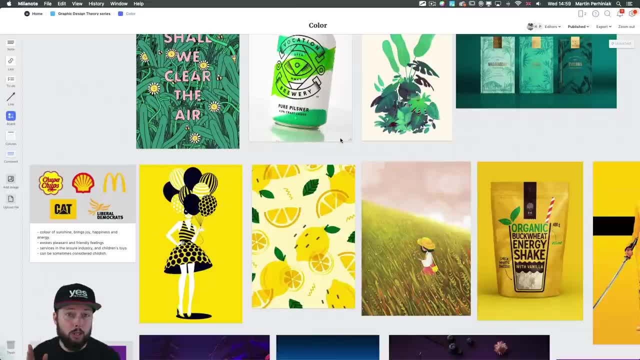 Now remember when we talked about value. amongst all the different hues, and yellow is one of the highest value color, So there is definitely a connection there why we would normally associate it with energy, But it is a color that is used for safety and for health, And it is also used for 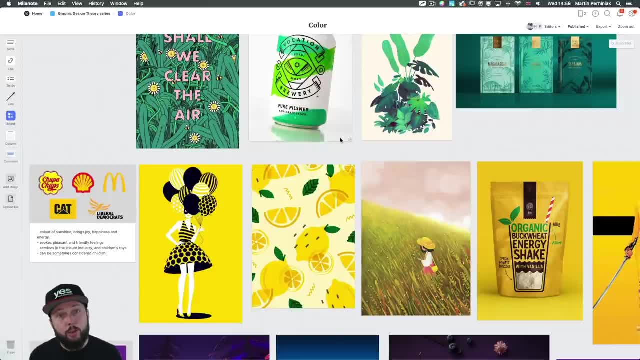 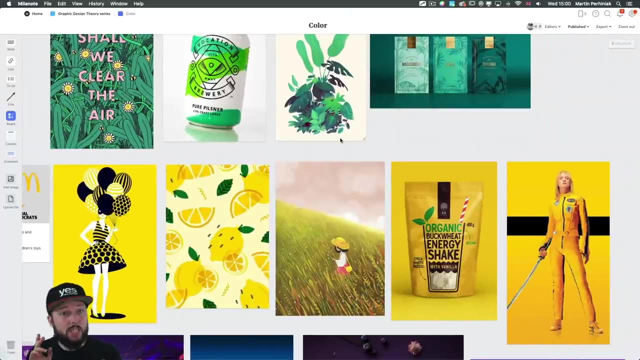 energy. Generally, when we look at yellow color, it evokes pleasant and friendly feelings And it's often used in the entertainment industry and for toys. However, that can also mean that sometimes it can feel a little bit childish. Of course, it didn't feel childish in Kill Bill, but you. 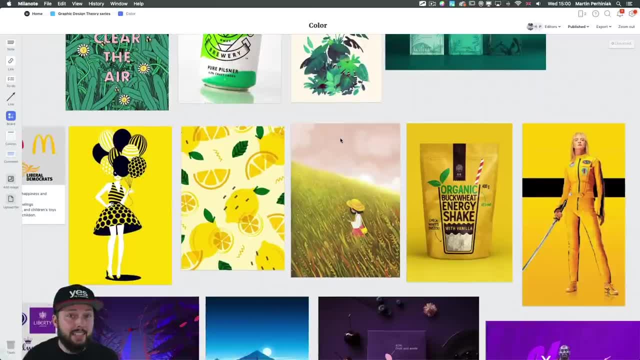 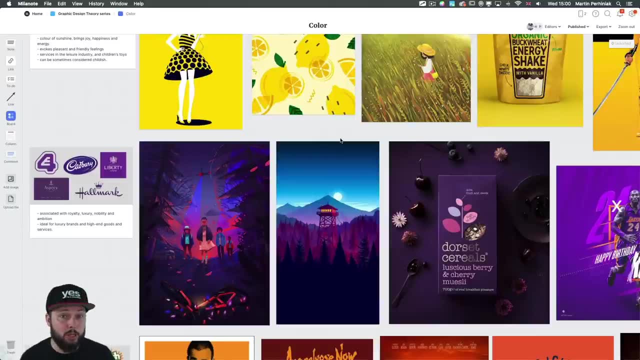 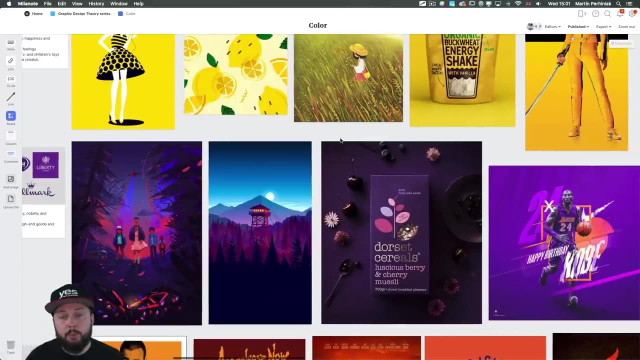 just have to be aware of that aspect of this color. Next, let's take a look at purple Now. this is usually associated with royalty, luxury, nobility and ambition, So it is ideal for luxury brands and high-end goods and services. It's worth remembering that purple is the least. 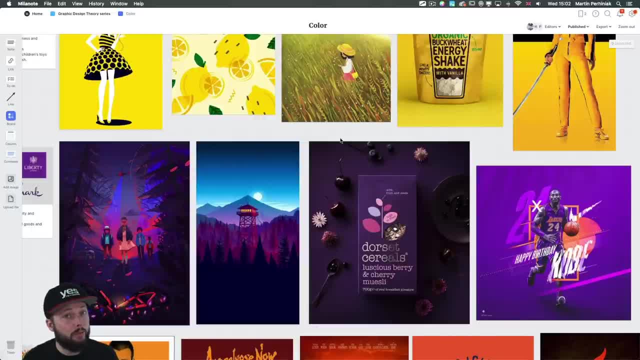 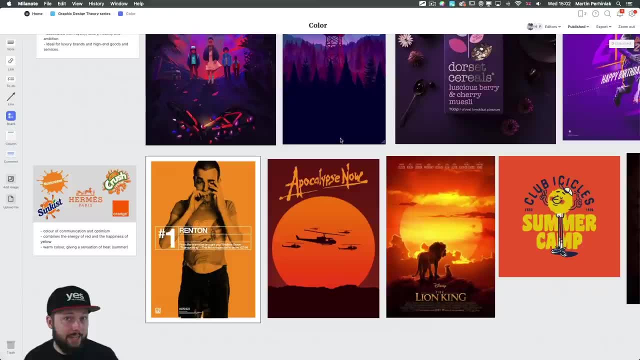 light color by men, But it is actually in the top three favorite color for women. And last but not least, let's take a look at orange. Now, this is the color of communication and optimism. It combines the energy of red and the happiness of yellow, And it usually can give the sensation of heat.